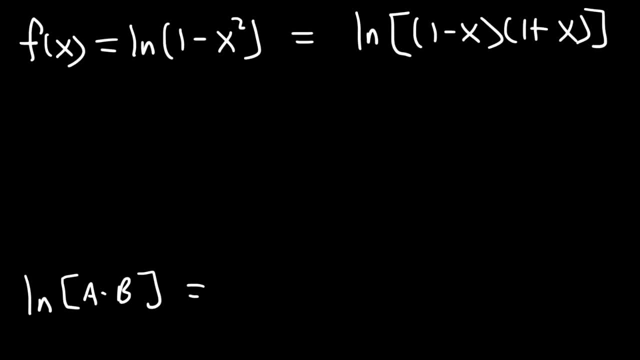 us to take a single log and express it as the sum of two logs. So ln a times b is ln a plus ln b. So therefore we can rewrite this expression as the natural log of 1 minus x plus the natural log of 1 plus x. Now here's a question for you. What is the derivative? 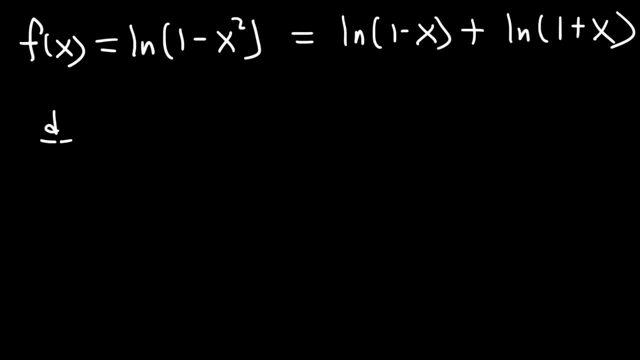 of ln, 1 minus x. So recall that the derivative of the natural log of u is going to be u prime over u. So in this case u is 1 minus x, So u prime, that's going to be negative 1.. So the derivative 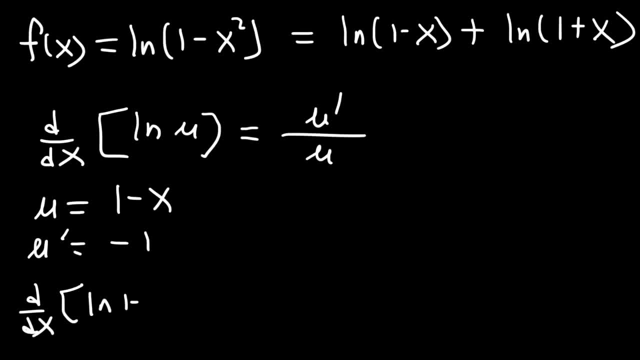 of ln 1 minus x is going to be negative: 1 over 1 minus x. Now what about the derivative of ln 1 plus x? So this is going to be 1 over 1 plus x. Now let's take the integral. 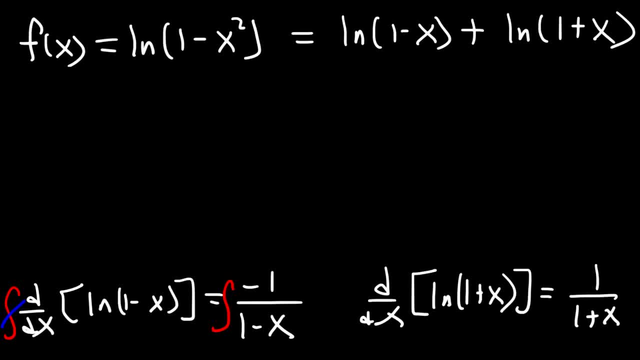 of both sides, These two will cancel. And so we can say that ln 1 minus x is the integral of negative 1 over 1 minus x, dx. And if we do the same thing here, we're going to get the same thing here. These two will cancel. And so we can say that the natural log of 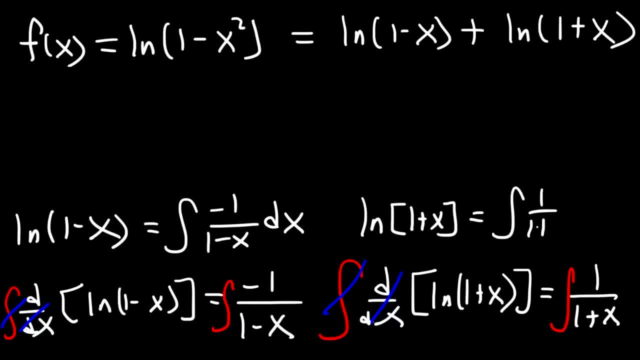 1 plus x is the integral of 1 over 1 plus x dx. So let's replace this with what we have here, And let's replace ln 1 plus x with this expression, And so this is all going to equal ln 1 minus x squared. 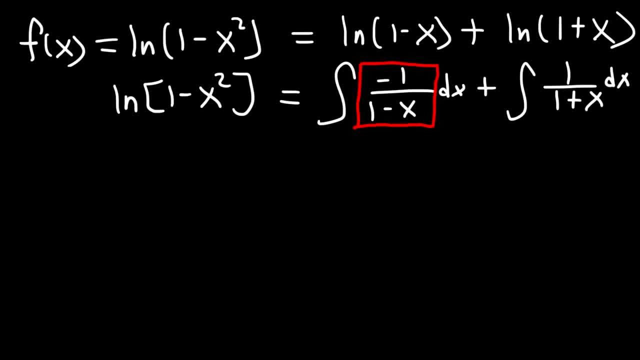 Now let's write a power series representation of negative 1 over 1 minus x, And let's do the same for 1 over 1 plus x. So this is all going to equal ln 1 minus x squared, And so this is all going to equal. 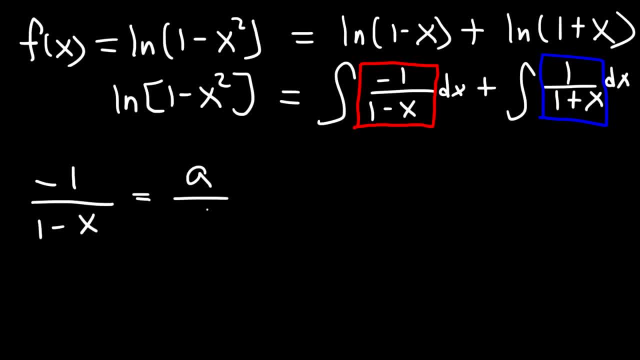 2 over 2 plus x squared. Let's rewrite the expression in a obvious form. What we're going to do in the form is we're going to charging these two figures now: 1 over 1 plus long mark, 1 over long mark. This is where any power can flow and traitthen Cartesian logarithm. 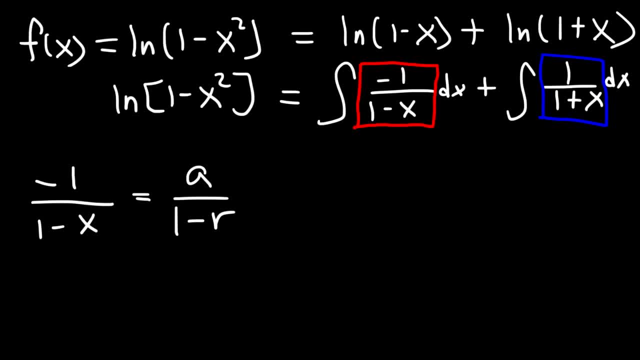 means health. So remember, refined Michael Jordan thought that this is area P over 2 to the power plus h times h squared. So do the same for the form A, WhenILL vs A. let's say here W is equal to F and Y is equal to an infinite geometric Tay ٩, and. 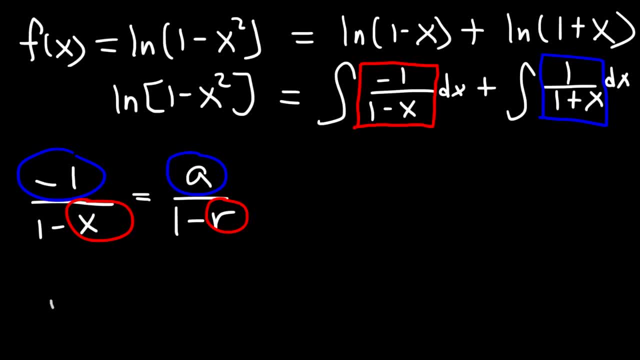 R is equal to a zero and P is PERFECT. So we find the sum of way V minus R minus Y times C, So we can see that A is 1, and R is x. Now, using the power series, I mean. 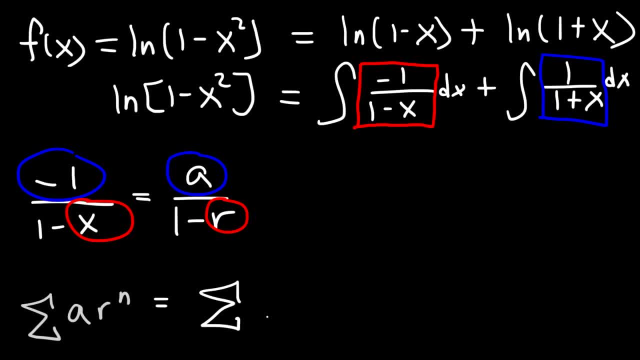 the geometric series. in that form We can write a power series like this: It's going to be a which is negative 1, times r, which is x raised to the n, from 0 to infinity. So we can say that ln 1 minus x squared is equal to this thing. but I'm going to write: 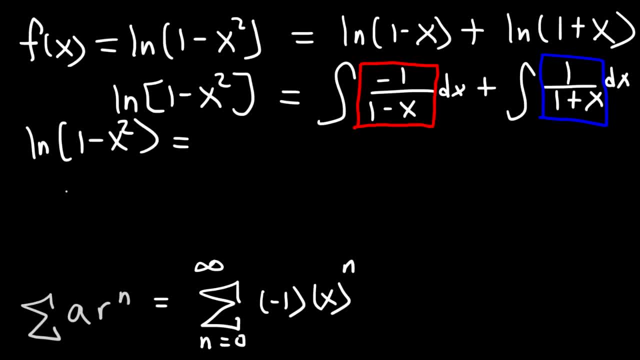 it later. Now let's focus on this one. We need to change the plus into a minus, so 1 plus x is the same as 1 minus negative x. So in this form we can see that a is 1, and r is negative x. 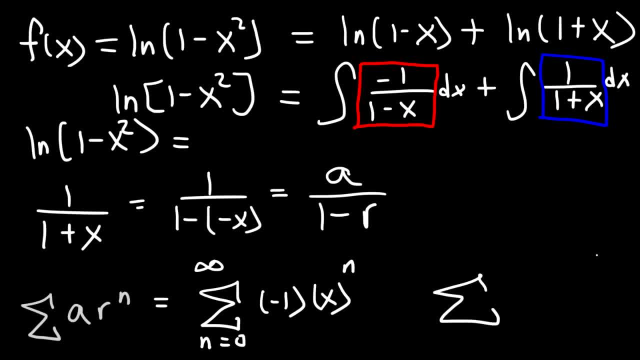 So using that expression we have the series 1 times negative x to the n, And negative x can be written as negative 1 times x, And all of this is raised to the n power. So if we distribute the n, we're going to get negative 1 to the n, x to the n, from 0 to infinity. 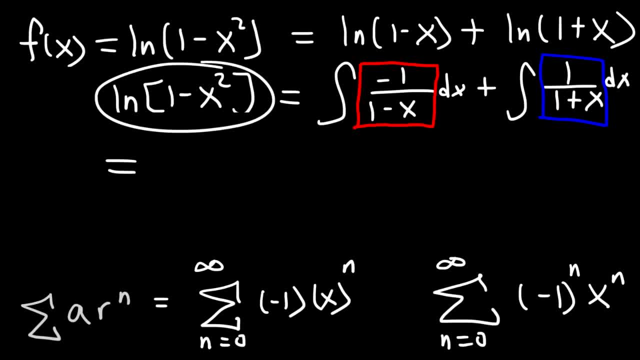 So at this point we can say that ln 1 minus x squared is equal to the integral Of this series. I'm going to move the negative sign to the front, And this is x to the n plus the integral of this series as well. 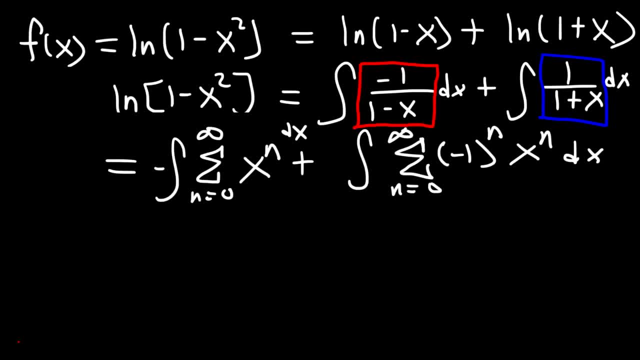 Now I'm going to combine these two integrals To one single integral. So we can say that ln 1 minus x squared is equal to the integral of the series from 0 to infinity. Now notice that we can take out x to the n. 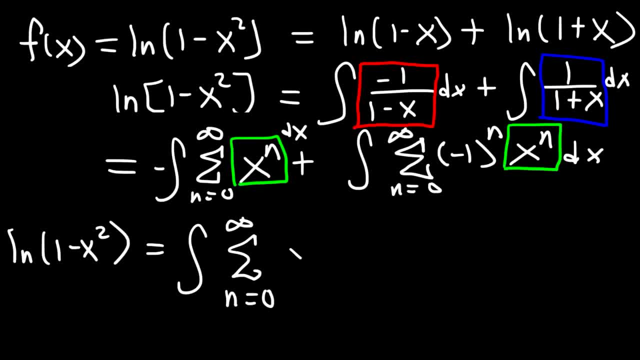 So that's a common factor that we can pull out, And then we're left over with negative 1 to the n, And then we have a negative for this one. So we can just say minus x to the n And then we have a negative for this one. 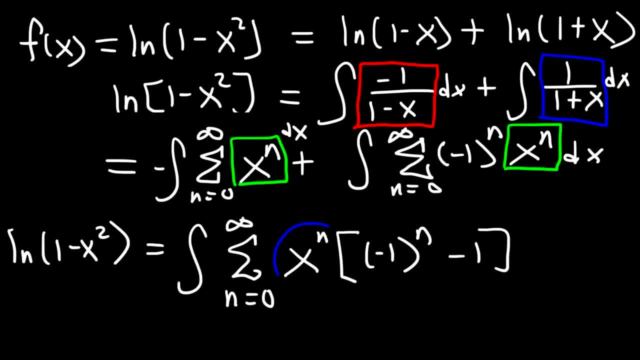 And then we have a negative for this one. So note that if I multiply x to the n times negative 1, it's going to give me that term, And then, if I multiply x to the n by this, I'm going to get this term. 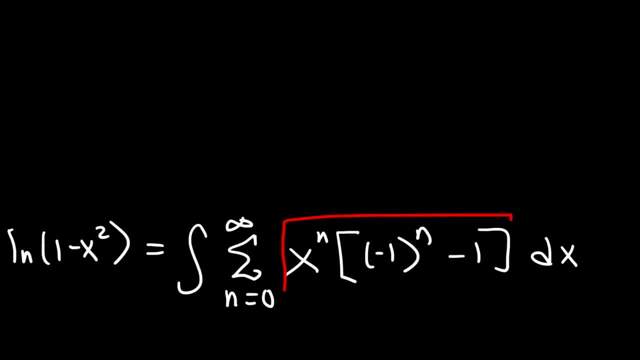 So what is the antiderivative of this expression? Now keep in mind: n is a constant, x is the variable, So this whole thing is a constant. Let's rewrite the constant first. So that's negative 1 to the n minus 1.. 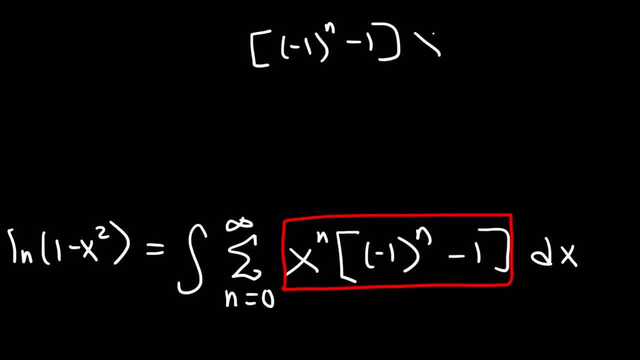 And then let's integrate x to the n using the power rule, So that's going to be x to the n plus 1, divided by n plus 1.. And so this is going to be the series from 0 to infinity, And we need to add the constant of integration plus c. 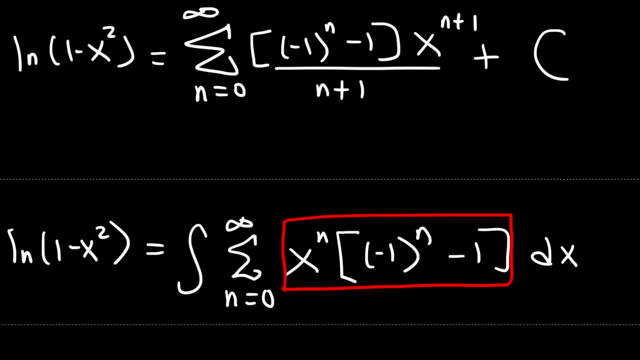 So now we have our answer. At least, this is one way of writing the answer. The next thing that we need to do is we need to calculate the value of c, the constant of integration, And so the best thing to do is to plug in: x equals 0.. 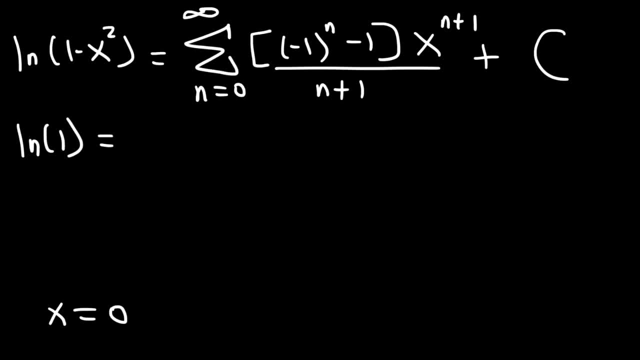 And so we're going to have the natural log of 1 on the left side, And on the right side this is going to be 0 to the n plus 1.. So 0 times anything is 0. And the natural log of 1 is 0. 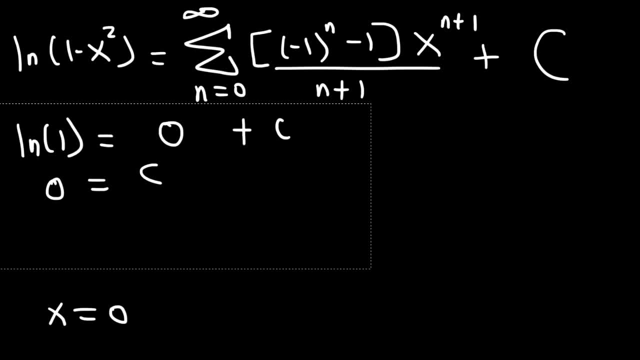 So 0 is equal to c. So we can get rid of this, And so we can say that the natural log of 1 minus x squared can be represented by this power series. Now there's more than one way to write a power series. 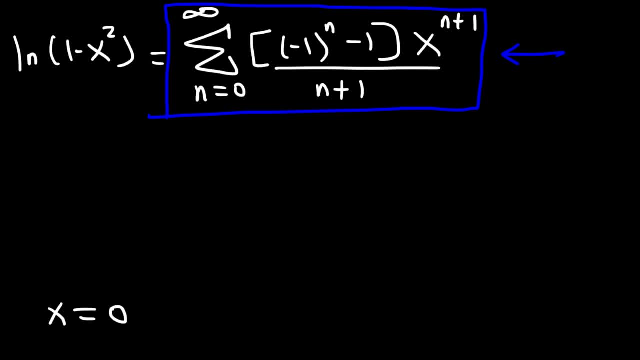 So can we write this series in a way that looks more appealing? Let's find out. So what we're going to do is we're going to write out the terms of the series. So let's start when n is equal to 0.. 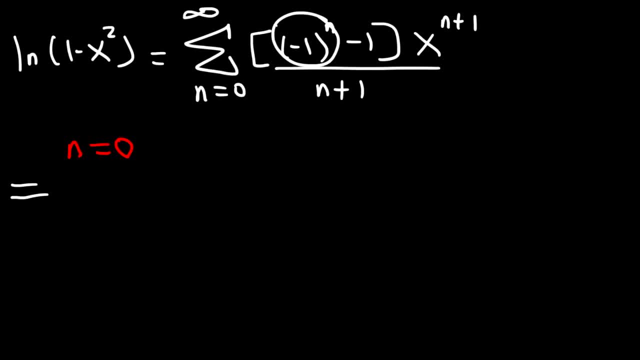 Negative 1 to the 0 power is positive 1.. And positive 1 minus 1 is 0.. Now, when n is equal to 1, this is going to be negative 1 minus 1.. And so we're going to get negative 2.. 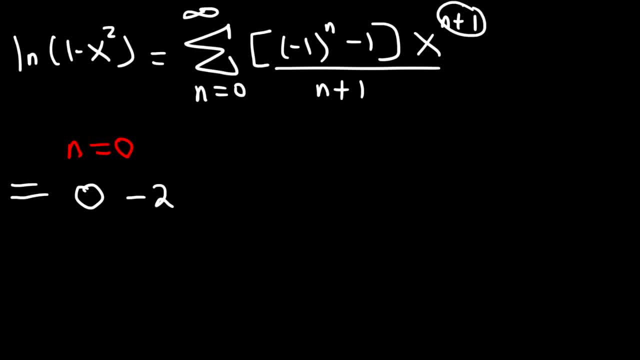 And then this is going to be 1. Plus 1, which is 2.. So that's x squared, And then this will be 2 as well. Now, when n is equal to 2, this is going to be negative 1 squared, which is positive 1 minus 1.. 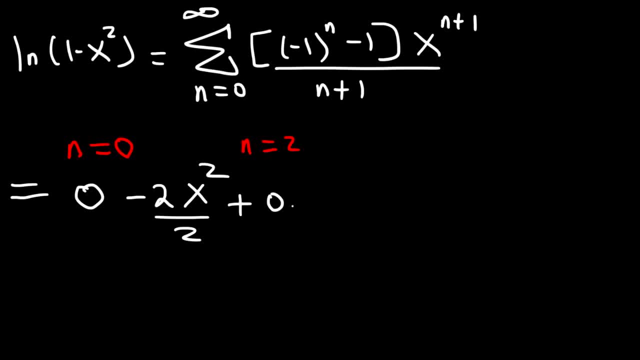 And so that's going to be 0.. So any time n is an even number, we're going to get 0.. Now, when n is equal to 3, this is going to be negative 1 minus 1.. And so that's going to be negative 2.. 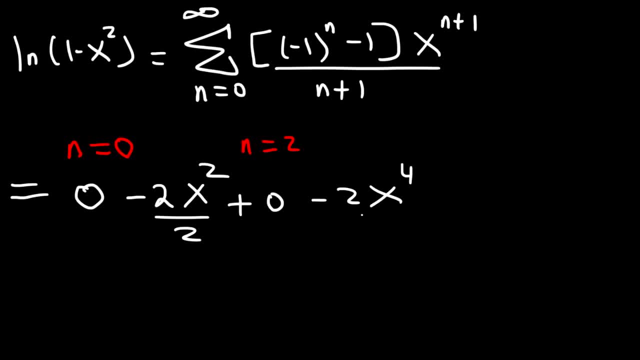 And then 3 plus 1.. 1 is 4.. So this is going to be 4 as well, And then it's going to be plus 0, minus 2x to the 6 plus 0. And then minus 2x to the 8 over 8.. 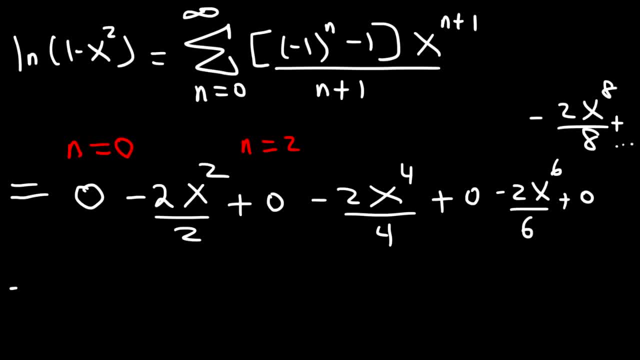 And then this will continue on forever. Now let's ignore the 0s, And what we're going to do is take out a negative 2.. And so we're going to get x squared over 2, plus x to the 4.. 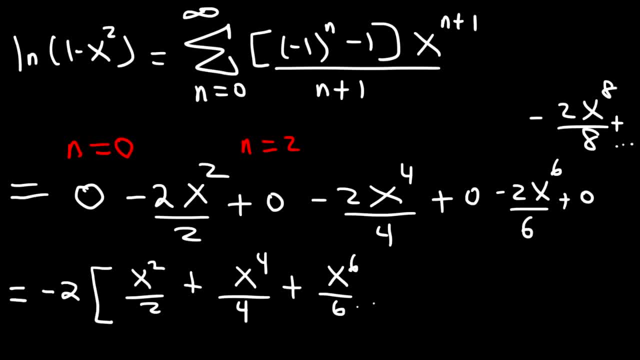 Divided by 4 plus x to the 6 over 6, plus x to the 8 over 8. And so forth. So what we're going to do is we're going to write a new series that corresponds to the numbers that we see here. 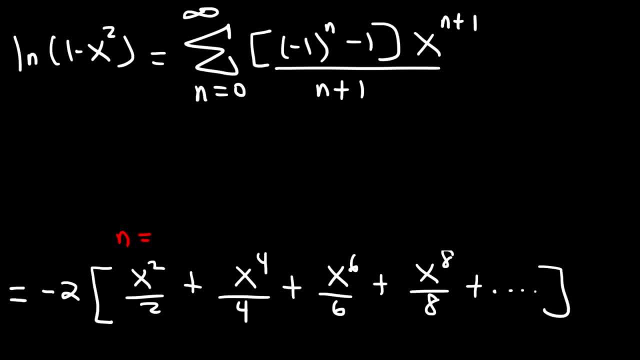 So we're going to say that n equals 0 for this term. Let me put it on. Let me put it on the bottom. And when n is 1, we need to get 4.. When n is 2,, we need to get 6.. 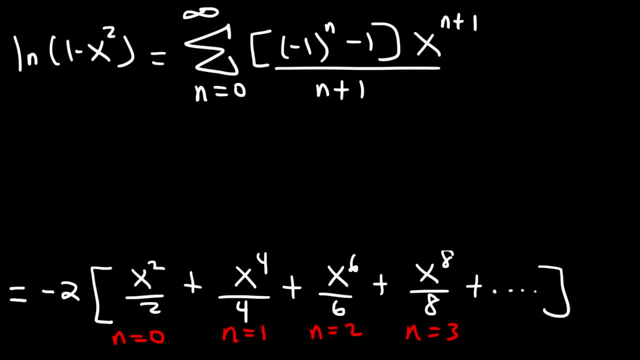 When n is 3, we need to get 8.. So how can we write a formula that corresponds to the arithmetic sequence 2,, 4, 6, 8?? We need to use this formula: a sub n is equal to a sub 1 plus n minus 1 times d. 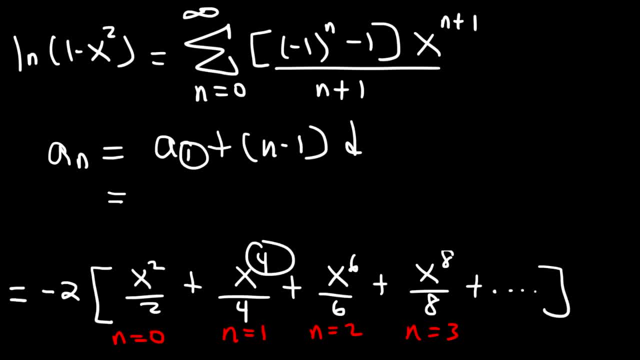 So when n is 1, we need to get an output of 4.. So we're going to say a sub 1 is 4.. And the common difference is 2.. Each of these numbers, they differ by 2.. And so this is going to be 4 plus 2n minus 2.. 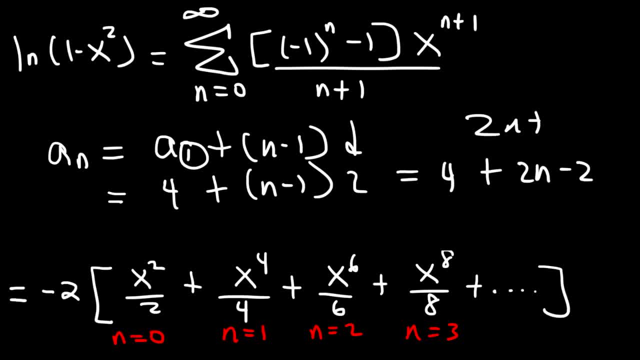 4 plus negative 2 is 2.. So we're going to get 2n plus 2.. So thus we can write this series like this: We could say: it's x to the 2n plus 2 divided by 2n plus 2.. 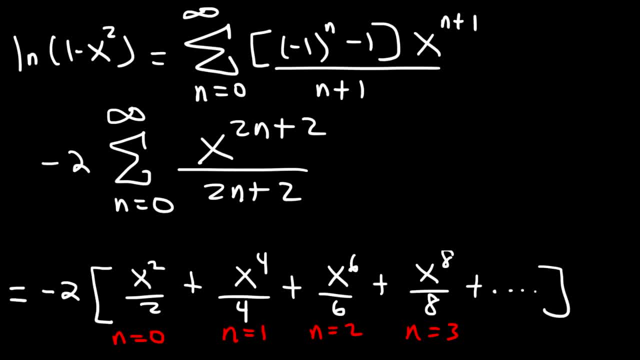 And we have a negative 2 in the front. So you could represent this function in any of the two ways, But this one is better because it doesn't include the 0 terms, which are just not needed. So this one is just more simplified. 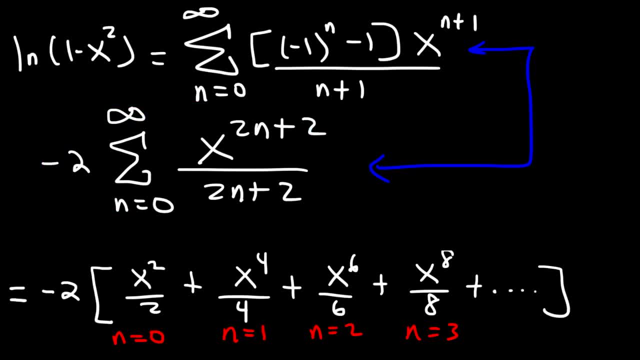 But both of them are correct. so keep that in mind. Now, what is the interval of convergence For this series? So keep in mind that series is based on the two geometric series that we had earlier in this video. In both cases, the common ratio is x. 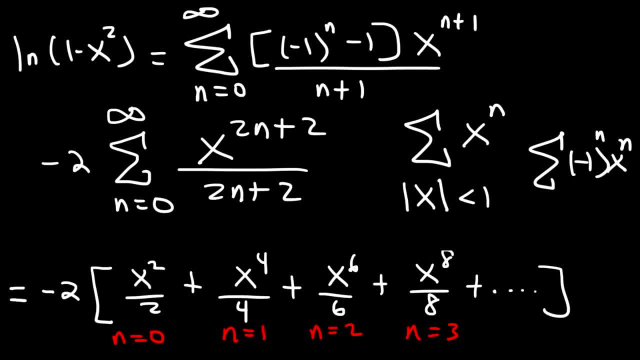 So x has to be less than 1, the absolute value of x for both of these two series that we combined to get this one before we integrated it. So for both of these series they will converge on this interval between negative 1 and 1.. 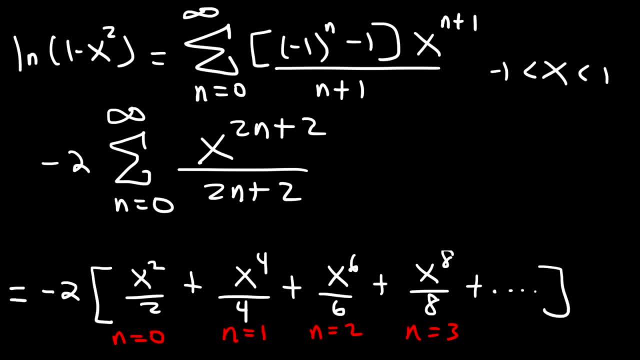 So when you integrate a series, the interval of convergence will be the same, with the exception that the endpoints may change. So if we were to plug in x equal 1 to this expression, we're going to have 1 over 2n plus 2.. 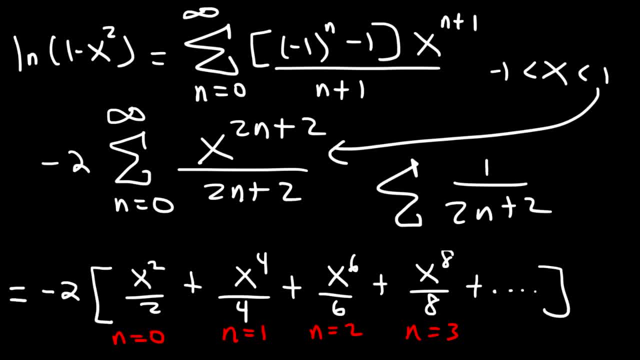 And will this series converge? No, Will this series converge when x is 1, or will it diverge Just by looking at it? if you take the, let's say, the integral test, it's going to diverge, And if you plug in negative 1,. 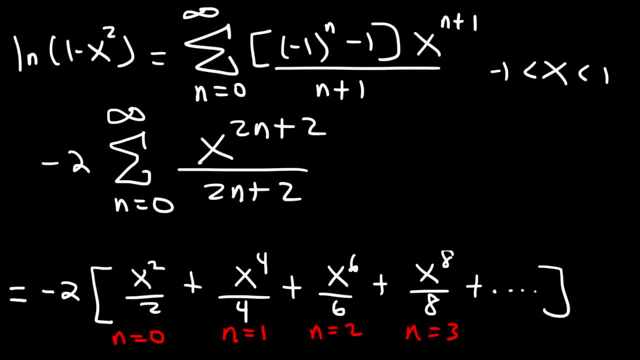 you're going to get negative 1 to the 2n plus 2, over 2n plus 2.. Now negative 1 to the 2n is the same as positive 1. And negative 1 squared is also positive 1.. 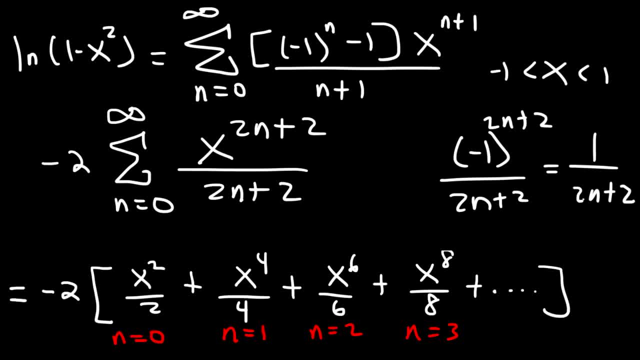 So this will be the same Using the integral test. that's going to diverge. Therefore, this function can be represented by this series only in this domain. Now let's make sure we have the right answer. So let's check the work that we have. 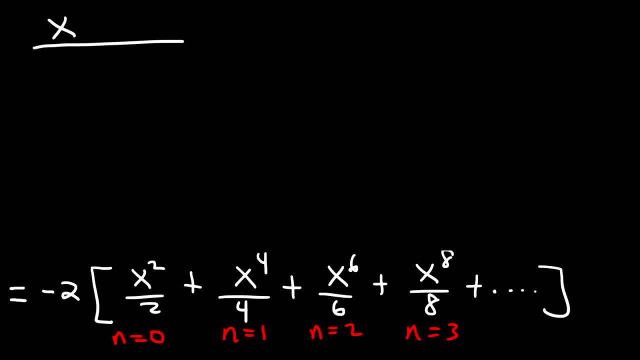 So I'm going to make a table. So this is going to be x and then ln squared and then the value that we get for the series. So let's try three points: 0.25,, 0.5, and 0.75.. 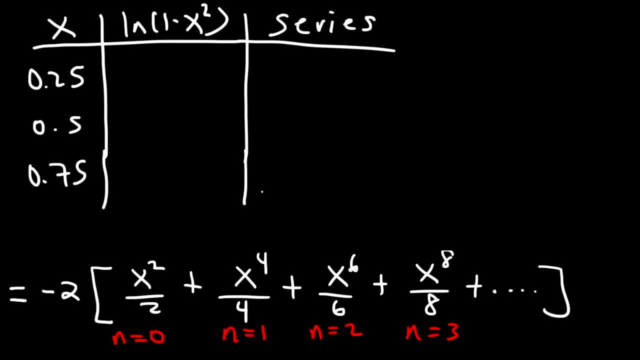 And notice what happens: The natural log of 1 minus 0.25 squared. if you plug that in, you should get negative 0.06454.. Now the natural log of 1 minus 0.5 squared, that's negative 0.2877.. 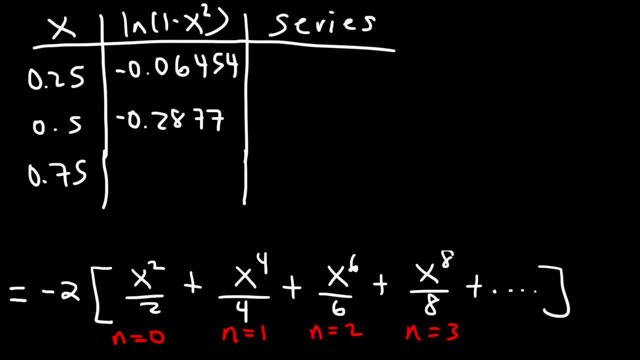 And then ln squared, that's going to be negative 0.8267.. Now let's see what we get if we use the series. So it's negative 2 times. the first one was x squared over 2, so this is going to be 0.25 squared over 2.. 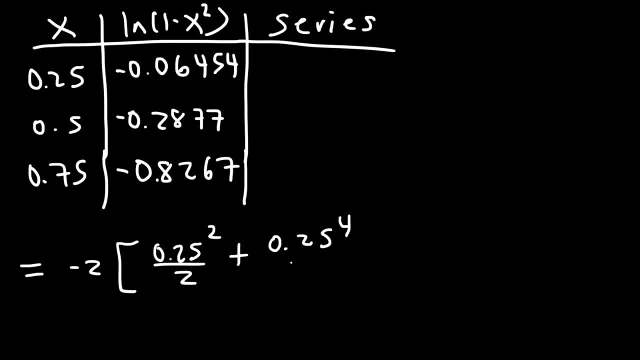 And then it's going to be plus 0.25 to the 4 over 4,, and then plus 0.25 to the 6 over 6,, and then 0.25 to the 8 over 8.. So we're going to stop at the first four terms. 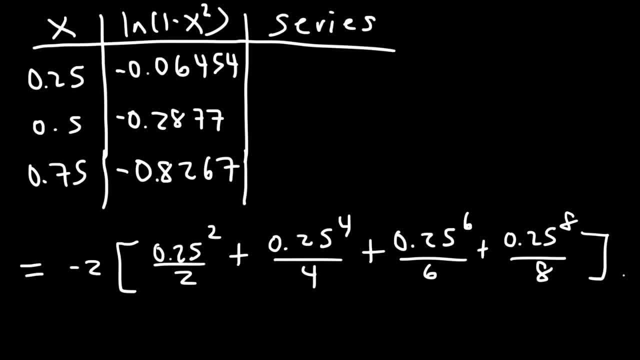 And we're going to see how good this approximation is. If we go on to infinity, it's going to give us the exact answer, But we're going to stop here, So go ahead and type this in And don't forget to multiply everything by negative 2.. 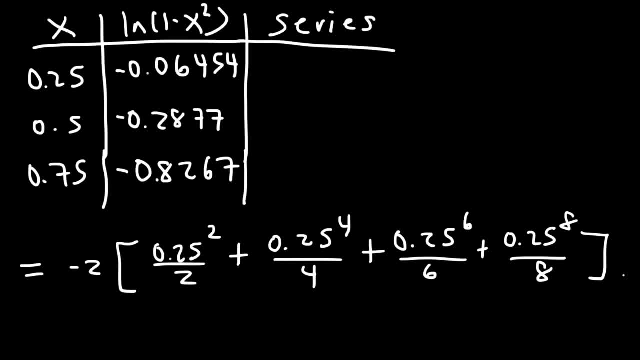 So you should get negative 0.06454.. Now go ahead and plug these values in as well, using the first four terms. So I got negative 0.2874, as opposed to 77. So it's a little bit different. 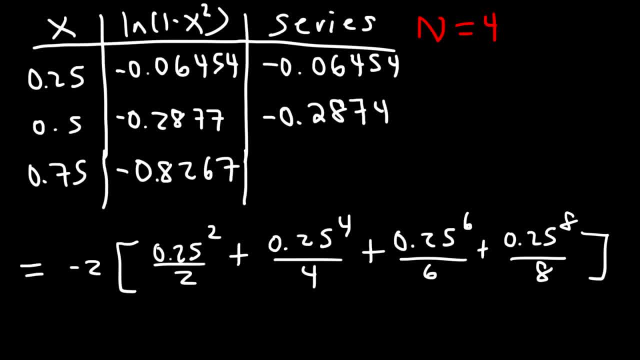 but it's still pretty close. Now let's do the same when x is 0.75 for the first four terms. So this is negative 0.8051.. So what do you notice is happening here as x increases from 0.25 to 0.75?? 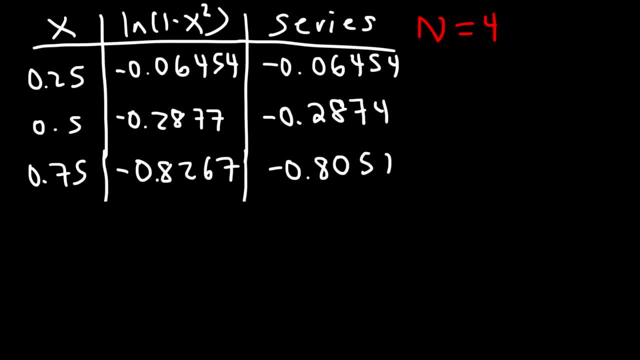 Notice that the accuracy decreases when n equals 4.. Now you can make this answer more accurate. You simply need to increase the n value. So if you add a few more terms, it will converge to this number. So the power series that we have is correct. 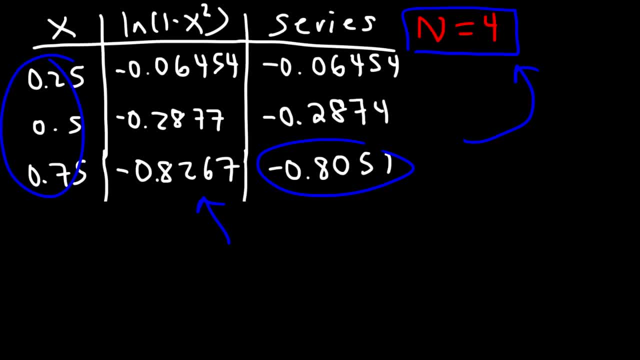 But let's talk about the trend that we see here and why that's happening. Now. we said that the interval of convergence it's negative 1 to 1.. And it's centered at 0 because 0 is the midpoint between negative 1 and 1.. 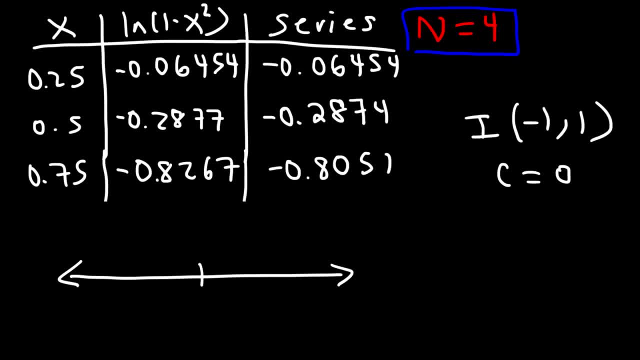 So let's plot the interval of convergence on a number line Now. the reason why it's so accurate at 0.25 is because 0.25 is very close to the center of where the series converges, And that is why we do not need to add so many terms.